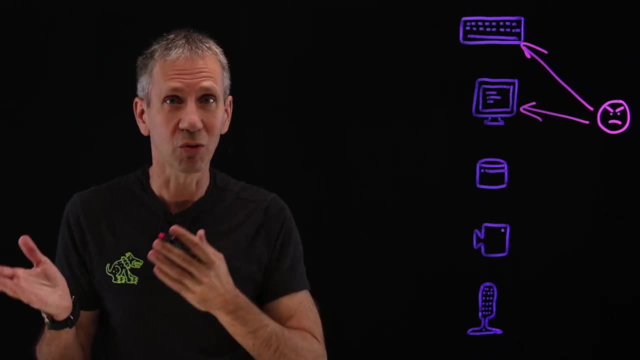 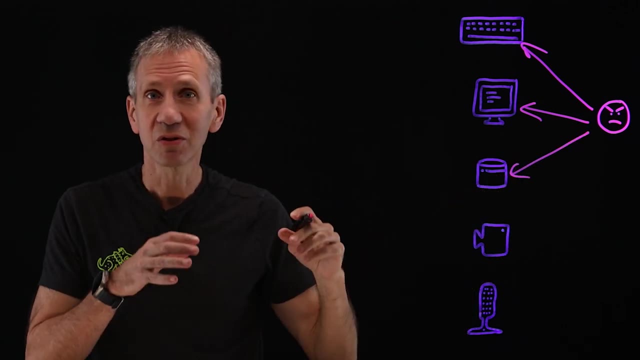 So all the sensitive, confidential information you might be reviewing, not only today but a week from now. he'll still be able to see everything that you see. He'll be able to have direct access to your disk. You'll be able to put malware on there, maybe ransomware, maybe encrypt all your files. 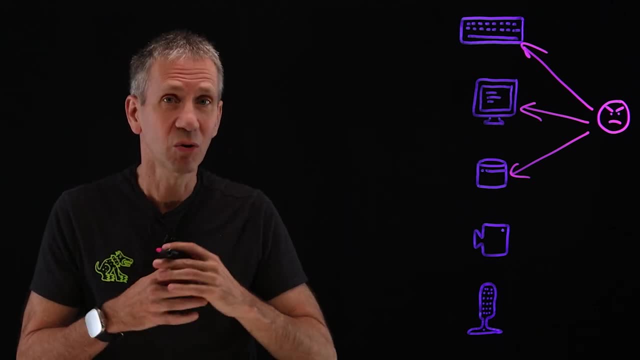 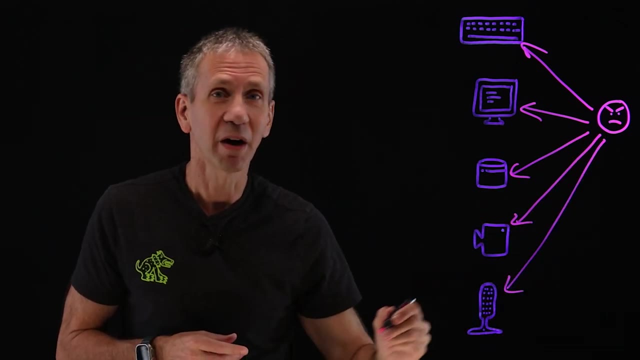 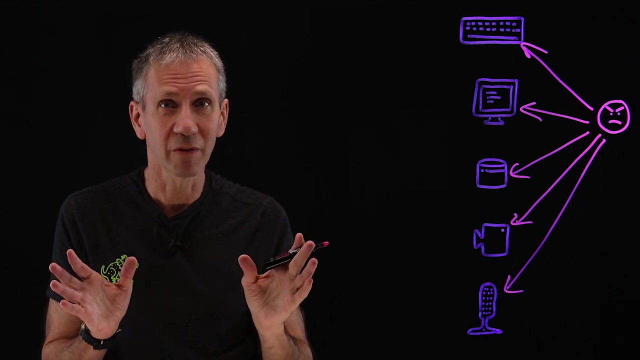 and make you pay him in order to get that information back Or just delete it all. He's going to have access to your webcam and to the microphone on your laptop. How about that, for creepy? In other words, he can turn these things on even when you're not aware of it. 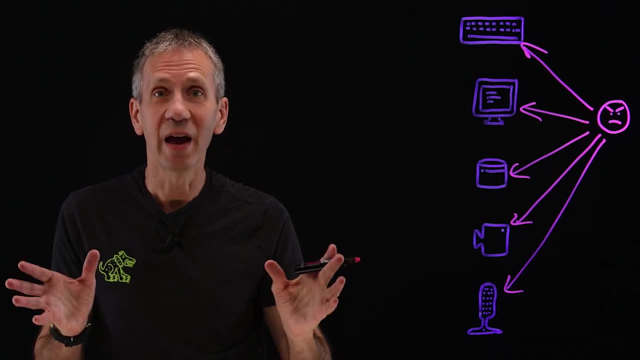 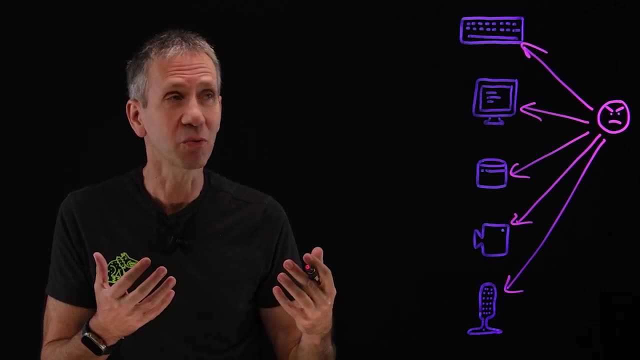 and see everything you do and listen to everything you say. That's what a remote access Trojan would do. There's other things called remote access tools that can be used by a help desk for legitimate reasons in order to do a couple of these kinds of things: to see what's working on your system and help you diagnose a problem. 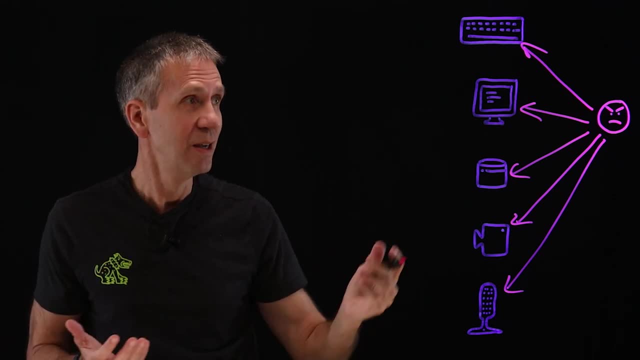 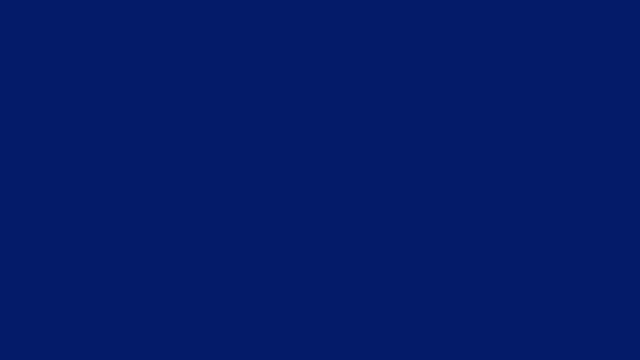 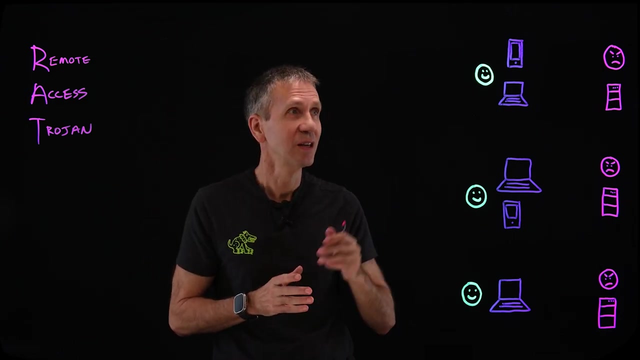 But in the hands of a wrong actor, this becomes a rat, a Trojan, and this guy has complete control over your system. Okay, let's see how these different types of infections can occur where you become infected with a rat. So the first one, we already took a look at. 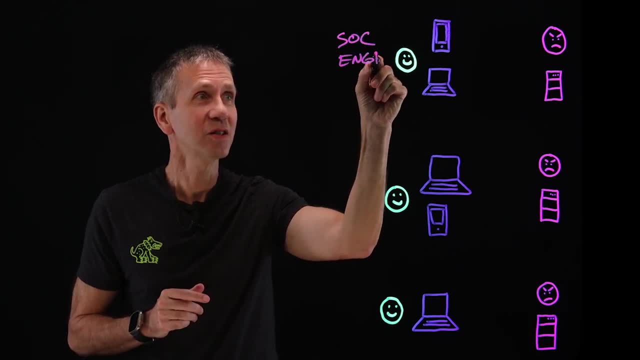 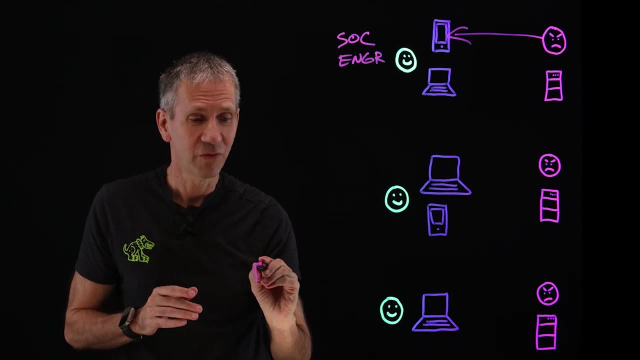 This is basically a social engineering attack And in this case, the bad guy is going to call this guy, And when he does, he's going to instill in him a sense of security, A sense of fear, uncertainty and doubt. FUD. 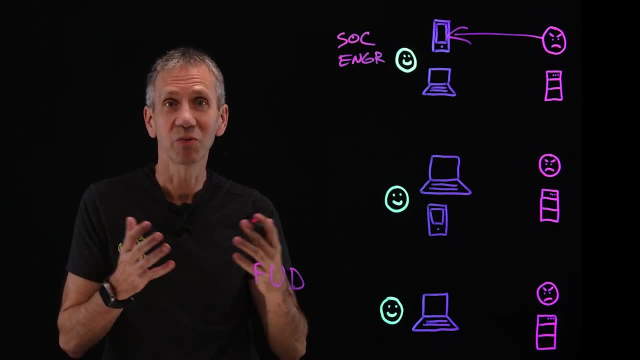 There's going to be a sense of urgency. You need to do something now, because we don't want you to stop and really think about this. We want you to just act, And what this guy is going to do is go onto his laptop. 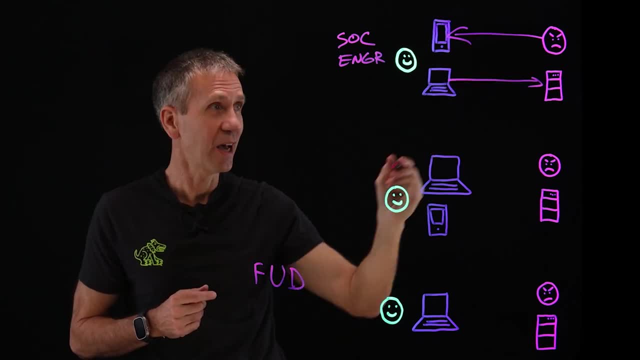 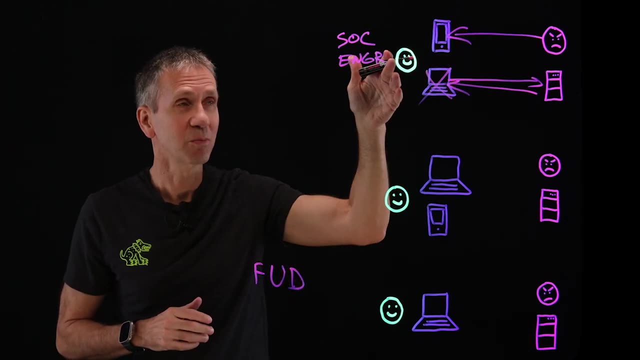 He's going to go over to the site that is controlled by the bad guy. He's going to download this stuff and now his system is infected with the rat, And this guy has complete control over his system. Let's take a look at another example. 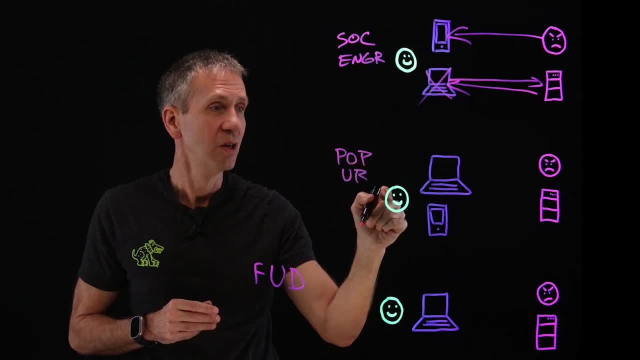 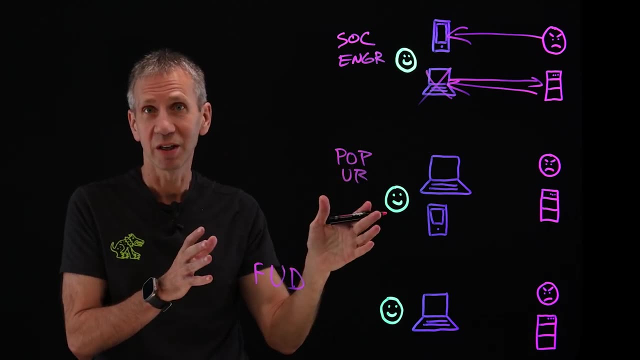 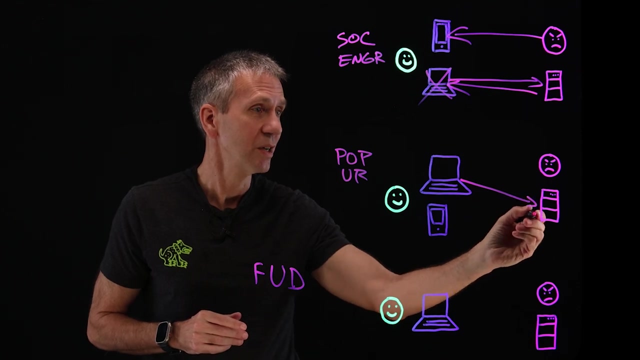 How about a pop-up? A pop-up occurs. This guy is on his laptop minding his own business, surfing the web, And all of a sudden a pop-up appears on his system And the pop-up gives him instructions. The instructions could be that he just goes to this site and downloads the disinfection software. 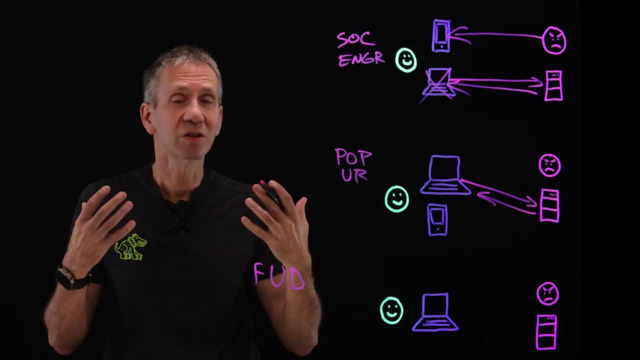 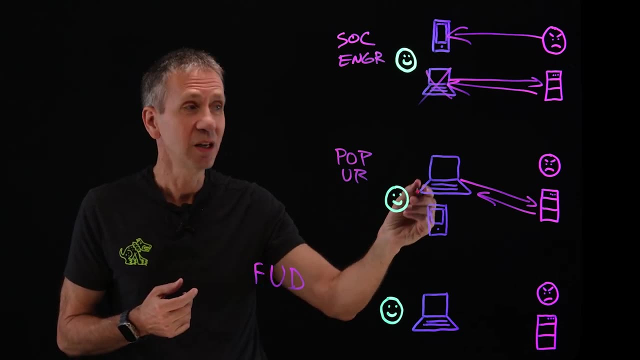 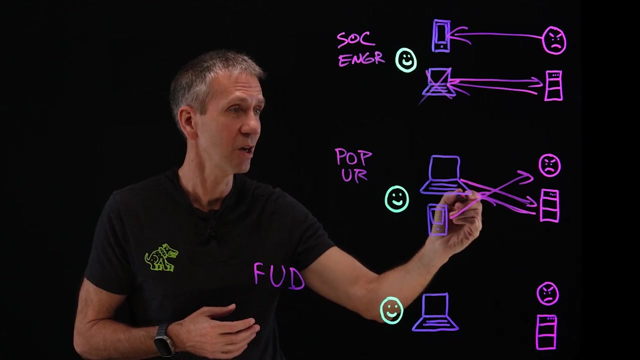 Because it's telling him you've got a virus- And, by the way, this is from some well-known antivirus company that it claims to be that it really isn't. It could be that it tells him to use his phone and call, And then the person he calls leads him through the same type of scenario. 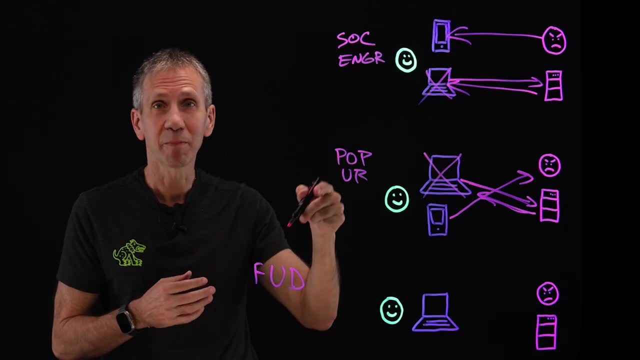 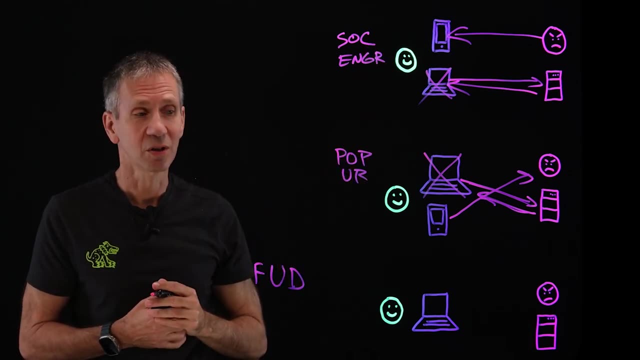 But the same results occur in both of these. The pop-up is just the way to initiate the action, But the user is actually infecting themself in both of these cases, And then one more that we'll take a look at is a more silent kind of case. 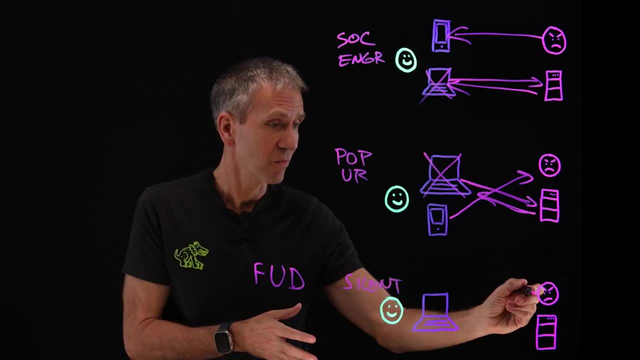 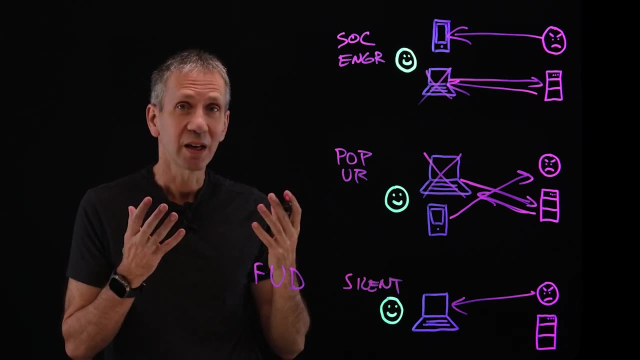 In this case, they're going to get an email. It's going to come from the bad guy And this email is like a phishing mail email or something of that sort, And it's going to tell him to click on a link. It may not tell him that he's been infected, or it might. 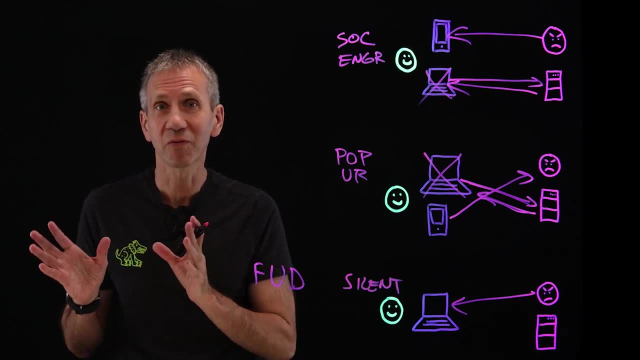 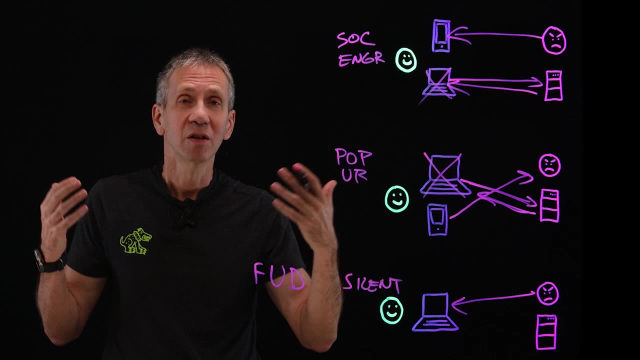 It could be either one of these circumstances. It could say that it's coming from his bank and he needs to install new software in order to access his accounts, Or it could say: we're from such and such antivirus company or such and such operating system company. 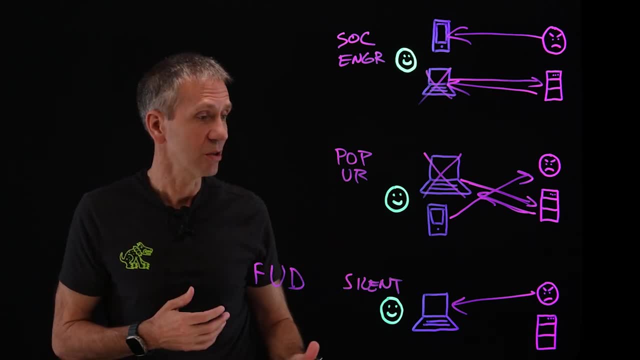 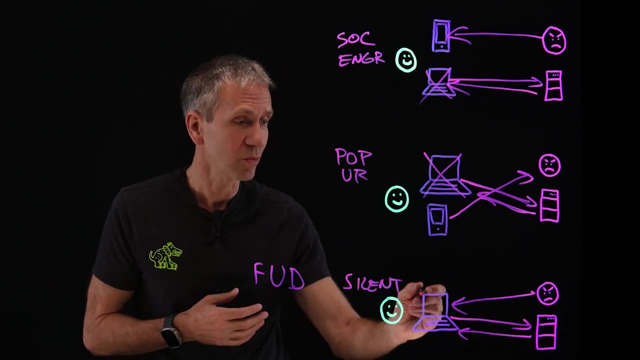 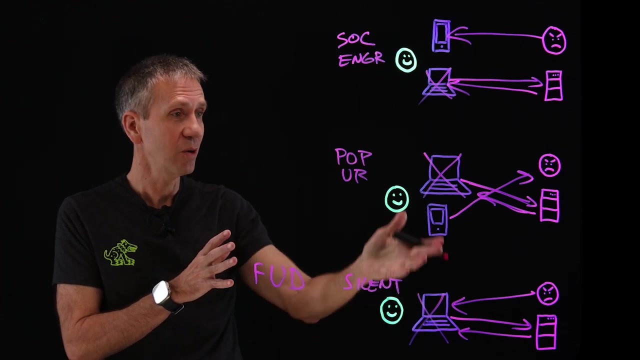 And we found the virus and we need you to install the software. Once again, same scenario. He goes over to the bad guy's site, downloads an app, downloads software and now he's under complete control. This guy now has a command and control server that allows him to do whatever he wants on the good guy's system. Okay. so what can you do to prevent this from happening to you? Well, there's a lot of things, in fact. That's the good news. First and most important, have a good backup. If everything else fails, you want to be able to go to your backup and recover. 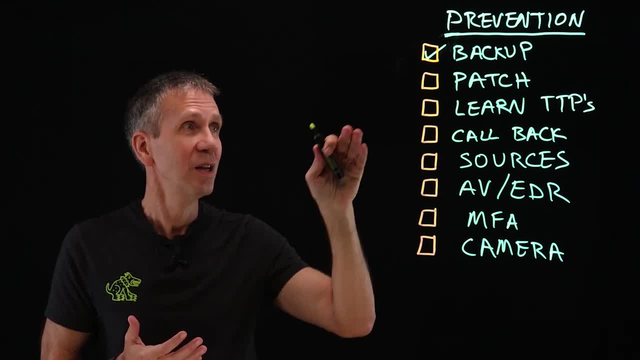 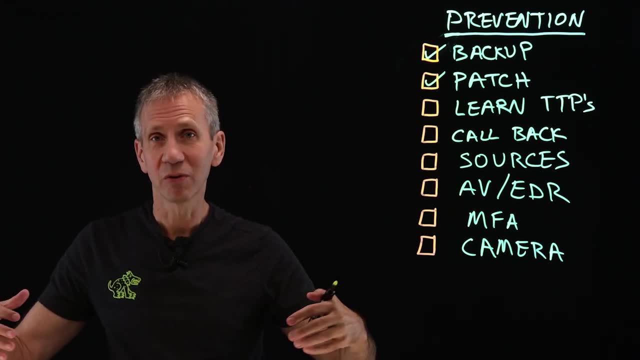 So make sure you have that. Do that now. Next thing is make sure that you patch your systems. I know it's inconvenient sometimes to stop what you're doing and put on all of those vendor patches from all the different apps and all the different OSs. 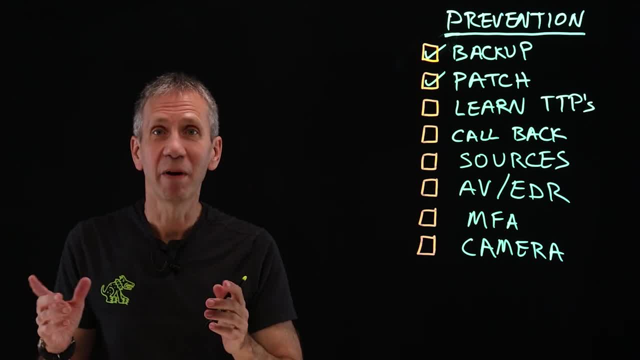 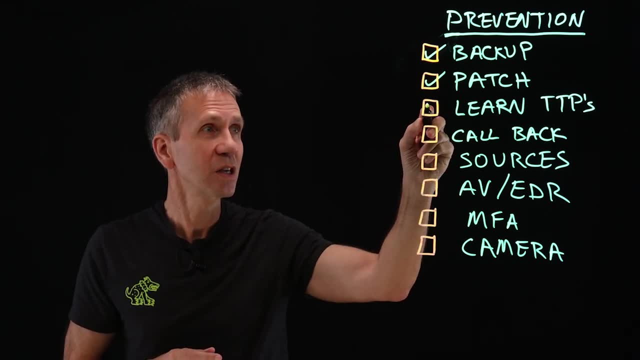 But if you don't, there may be a vulnerability that the bad guy is going to exploit that gives him the remote access Trojan capability onto your system. Another one is: learn the tactics, techniques and procedures of the bad guys. In other words, how do they go about doing what they do? 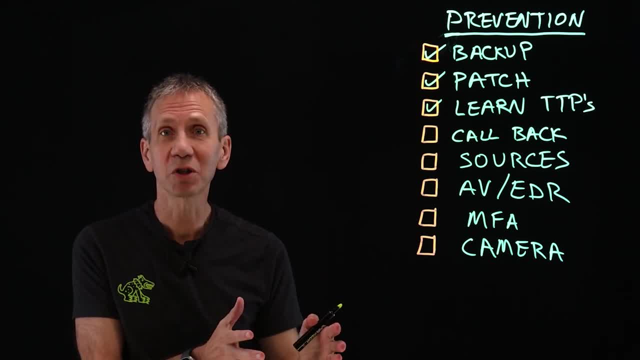 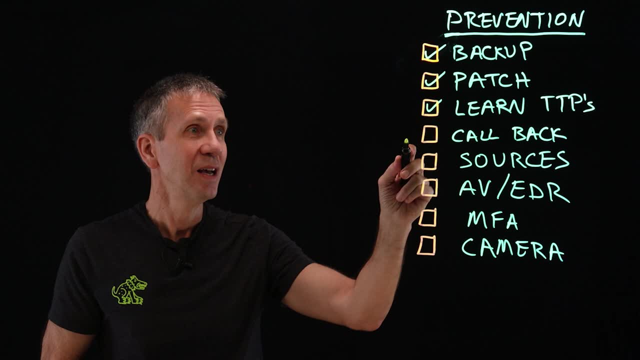 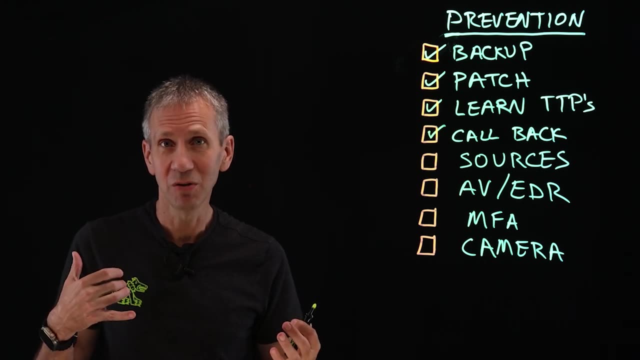 If you understand how your adversary works, then you'll have a much better idea of how to avoid what they do And you won't fall victim to it. So be aware, Educate yourself. Then, if you do think you need to call tech support for a problem, if they call you and report that they found an issue. 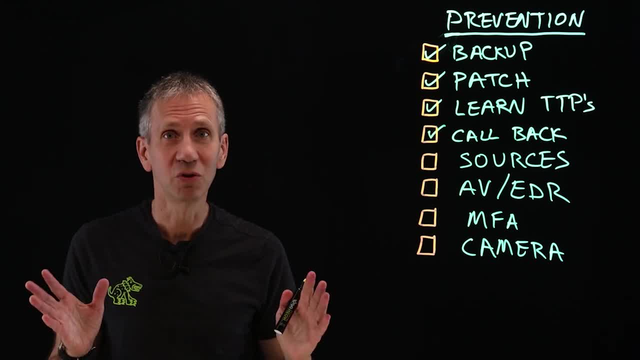 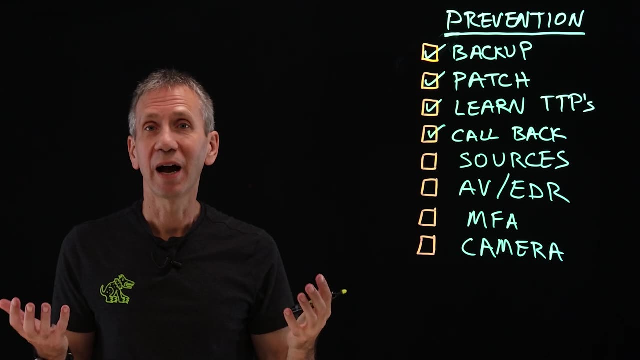 I'm going to tell you. first of all, generally, operating system companies do not call customers out of the clear blue, So you should suspect that something is up. Neither do application vendors, for the most part either. So if you do think for some reason you want to check this out, say okay, I'll give you a call back. 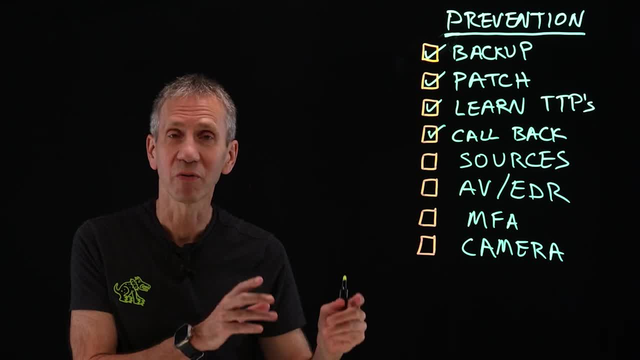 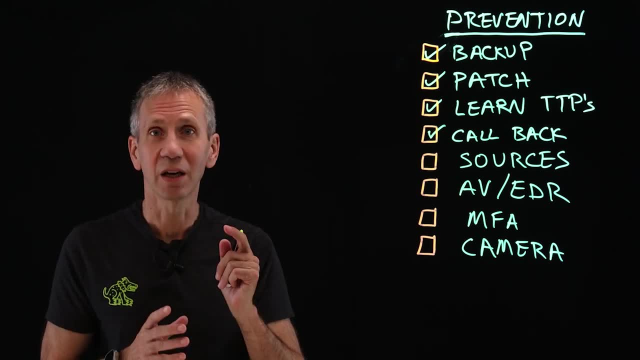 And don't take the number that they tell you. Then you go and look up the number for that company and you call them directly And then you can find out. So you do a separate call that you've initiated and you know where you're actually calling. 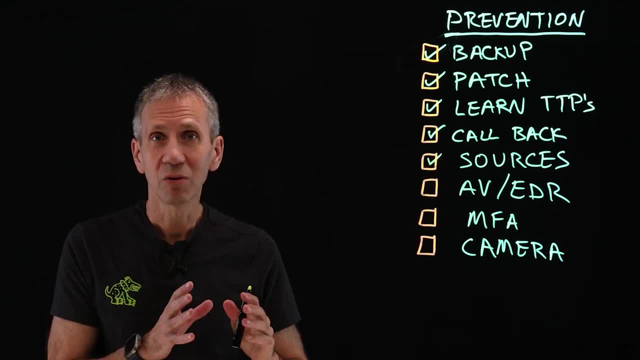 Get all of your software from trusted sources. Don't go to just any old app store and download stuff, because that may have a Trojan inside of it And you may have just infected yourself. So, as best possible, know that your software comes from trusted sources. 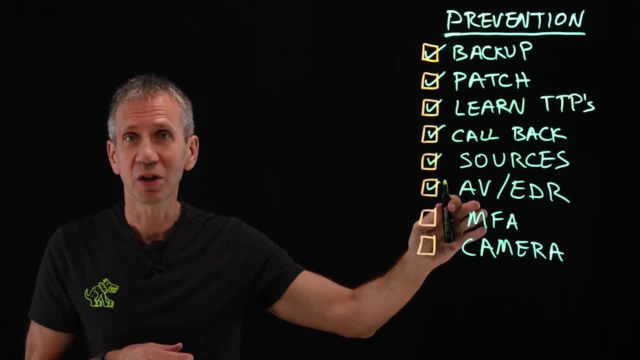 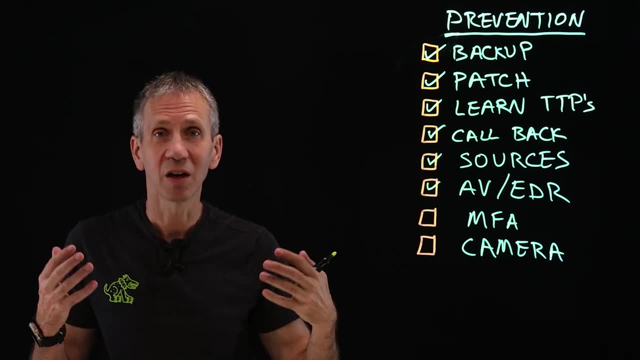 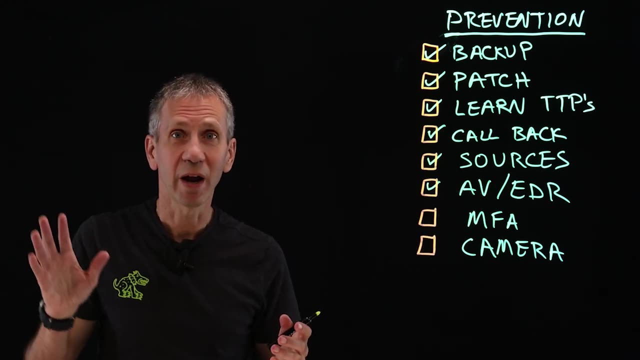 Use antivirus in-point detection and response software. The EDR stuff is used more in enterprise environments, AV very common on user retail systems. But use these technologies because they can sometimes detect these rats, the well-known ones, and stop them in their tracks. 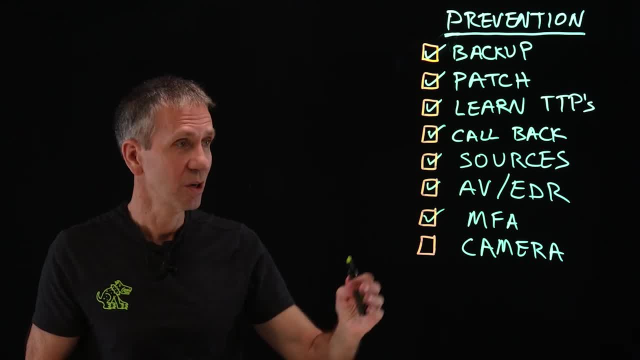 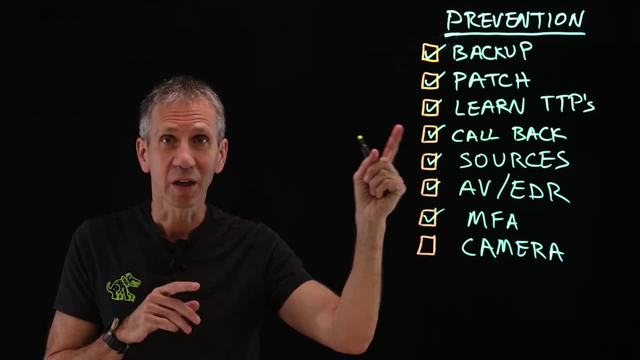 And then, as another tip, another sort of safety measure, use multi-factor authentication on all of your accounts. Don't let it just be a user ID and password that gets you in, because the guy controlling the rat may remember control your keyboard. 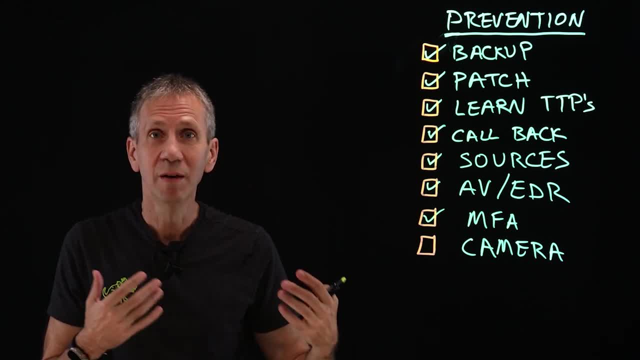 And when you type in your password they get your password, Then they can log in as you. But if they also need to have possession of your phone in order to get your biometric, to open the phone up or to get into the app, you know with an SMS message that goes to your phone. 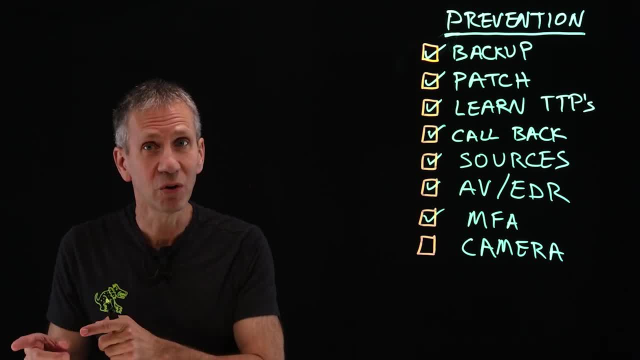 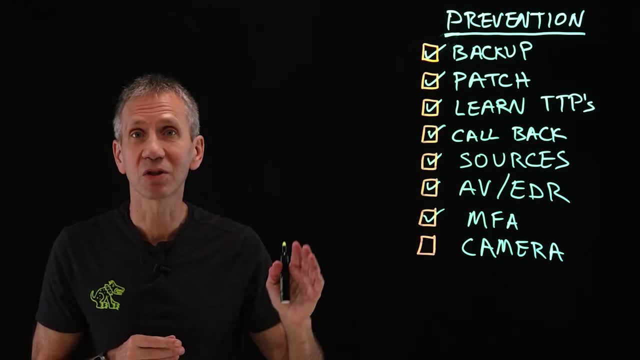 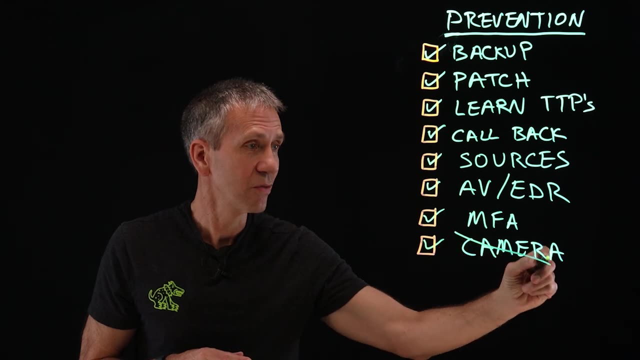 it makes it harder for them. Of course, they could have a rat on your phone as well, So there's a lot of different things that could be involved here, But multi-factor authentication certainly makes the job harder for the bad guy, And then one of the other things you could do is basically turn off the camera or put a block.